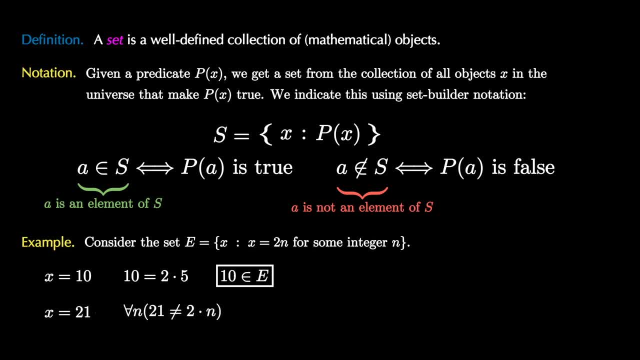 x equals 21,. we see that twenty-one is not twice any integer, and therefore 21 is not an element of e. Let's check a couple more. Let's consider the real number. x is pi. This is not twice any integer either, and therefore pi is not an element of E. 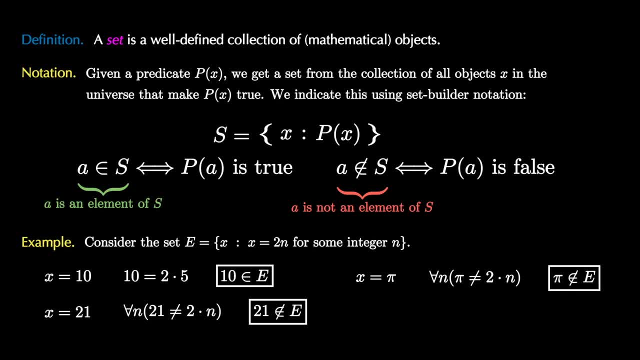 Finally, a number like x equals 208, is 2 times 104, and 104 is an integer, so 208 is an element of E. Total consideration of the set E shows us that the set E is the set of all even integers. 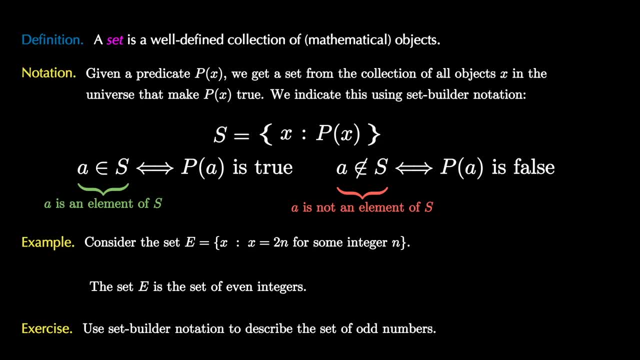 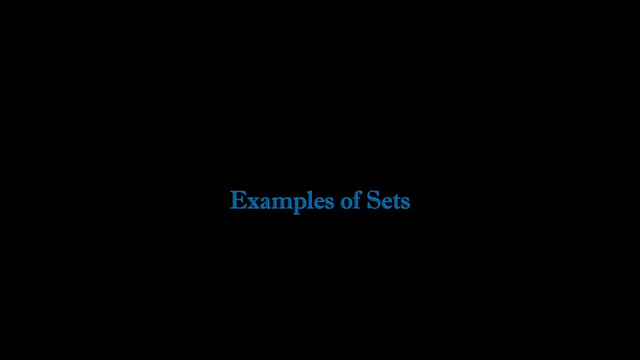 Try this out yourself. Use set-builder notation to describe the set of odd integers. Let's look at some examples where you've used sets before but might not have used set-theoretic notation. When studying Algebra and Mathematics, it's important to remember that the set E is the 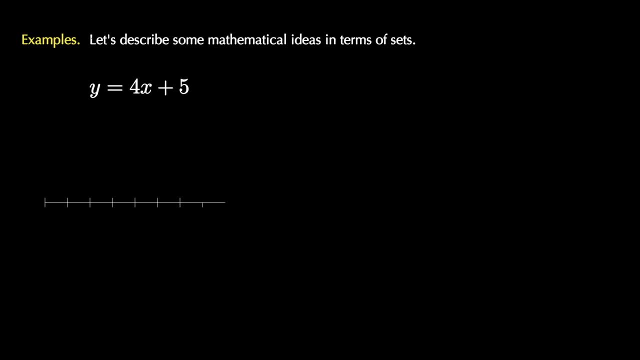 set of all, even integers. In pre-calculus you often look at equations like y equals 4x plus 5.. Typically the idea is to graph this equation to see that it looks like a line, But really what you're doing is you're looking at a bunch of ordered pairs of dots. 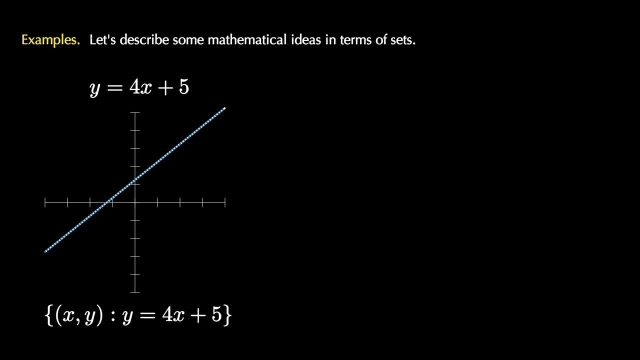 in the plane, these blue dots, and it turns out that they all lie along the line. So what you're really doing is you're graphing the set of ordered pairs of the form x, comma, y, such that the equation y equals 4x plus 5 is true. 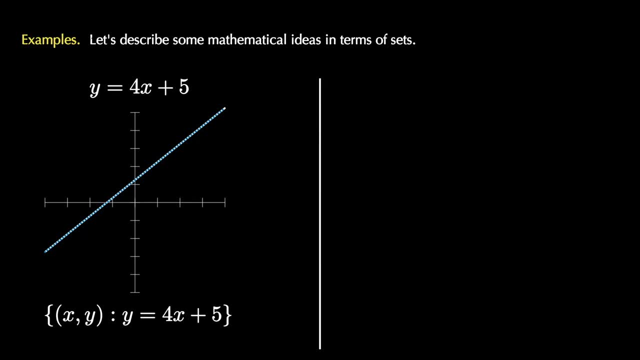 That means the equation y equals 4x plus 5 becomes the predicate of the set in question. Another algebraic question is to solve the equation x, squared minus 5x plus 6, equals zero. We know this has a graphical interpretation, but what we're looking for is we're looking 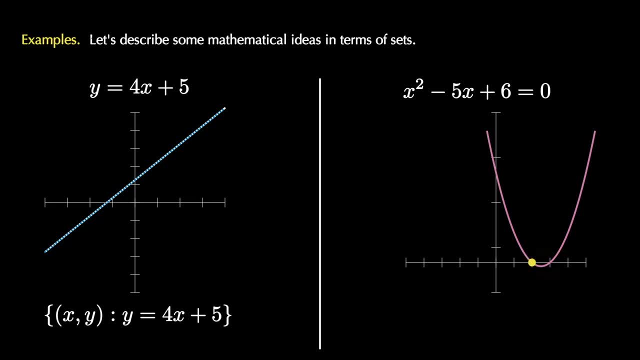 for the x values where this graph crosses the x axis, We see that there are two such points. Therefore, we're looking for the collection of all x, such that x, squared minus 5x plus 6, equals zero. And in this case, we're looking for the collection of all x, such that x, squared minus 5x plus 6, equals zero. 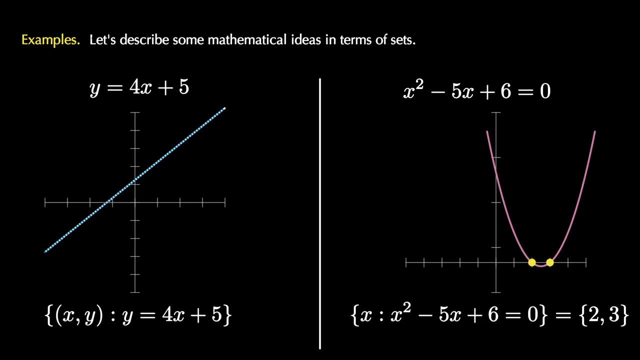 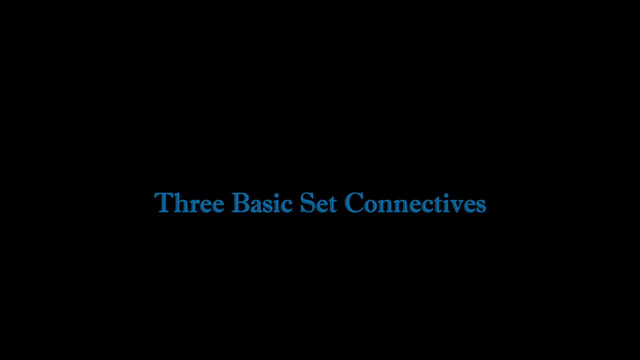 In this case, this is just the set containing the numbers 2 and 3.. Since sets are built from predicates and predicates are related to propositions, it makes sense that there will be set-theoretic interpretations of the logical connectives. Let A and B both be sets. 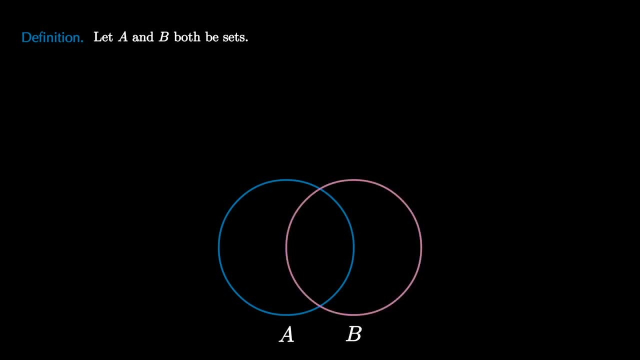 We can depict A and B with circles that are labeled by the appropriate letter. Now we can create new sets using three elementary set connectives. First, the union of A and B. A and B denoted A. union B is the collection of x, such that x is in A or x is in B. 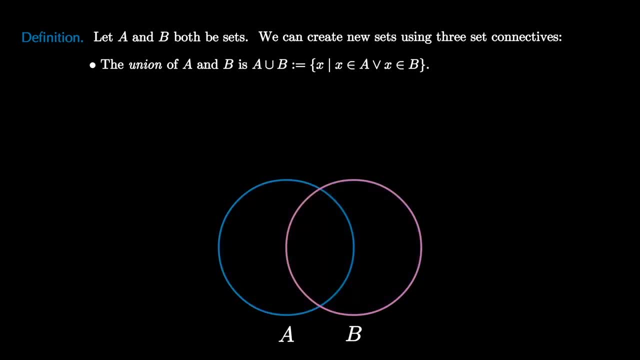 This is the set-theoretic interpretation of the or statement. Next is the intersection of A and B, denoted A intersect B. This is the collection of x, such that x is in both A and B. This is the set-theoretic interpretation of the and statement. 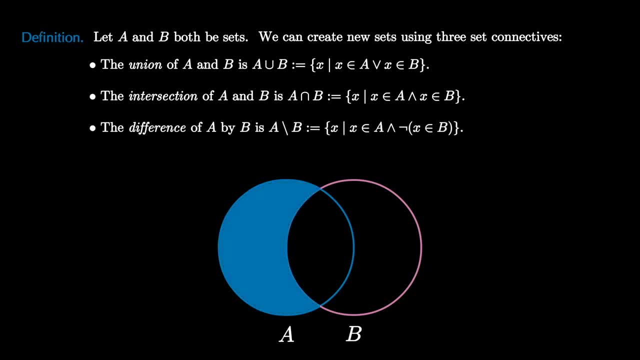 And the final elementary connective is the difference of A by B, denoted A set minus B, Which is the collection of x that are in A and not in B. This is the set-theoretic interpretation of the and statement. And the final elementary connective is the difference of A by B, denoted A set minus B, which is the collection of x that are in A and not in B. 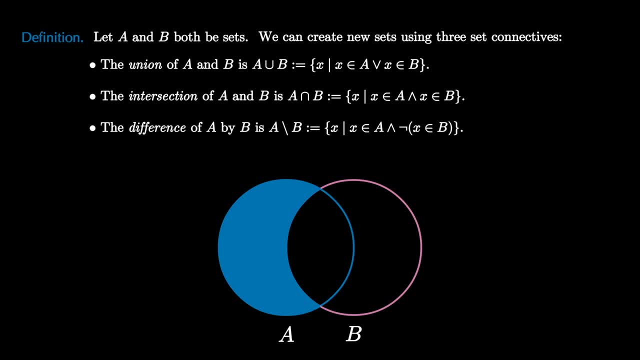 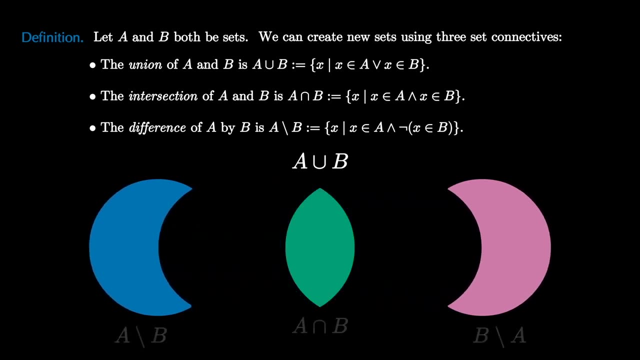 in B, pictured on the left. here You can think of this as the collection of things that are only in A and not in B. As a final note here it's interesting to see that the union of A and B can be split into three pieces that have nothing in common. On the left we have the set A set. 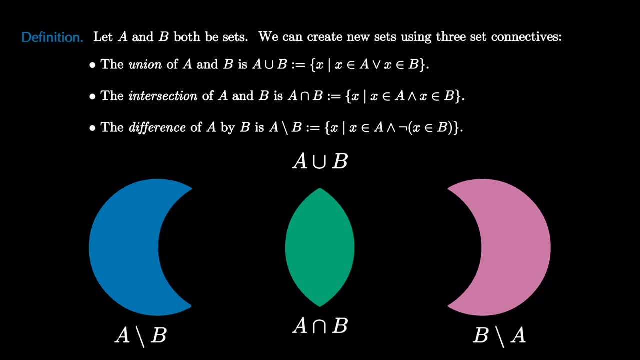 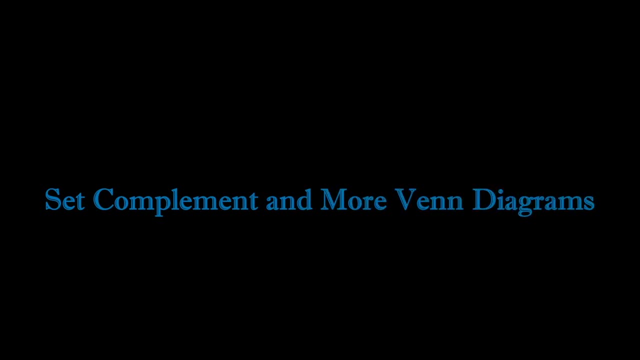 minus B. In the middle we have A intersect B and on the right we have B set minus A. Therefore, A union B is the union of these three sets, and none of them have anything in common. We call this a disjoint union. Let's look at one more set operation as well as the Venn diagram for 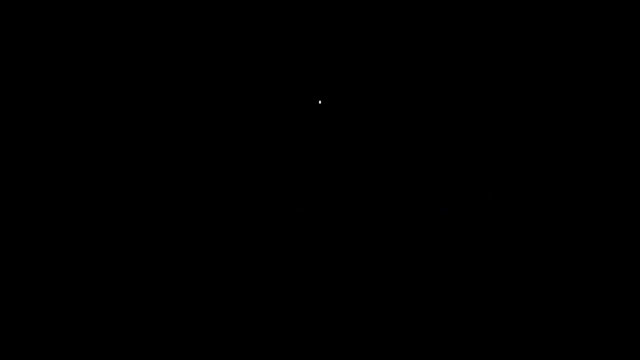 three sets. The different set connective is strongly related to the not connective from logic. The complement of a set A in a universe U is the collection, A bar, which is the set. U set minus A. This represents the collection of all the things that are in the universe and not 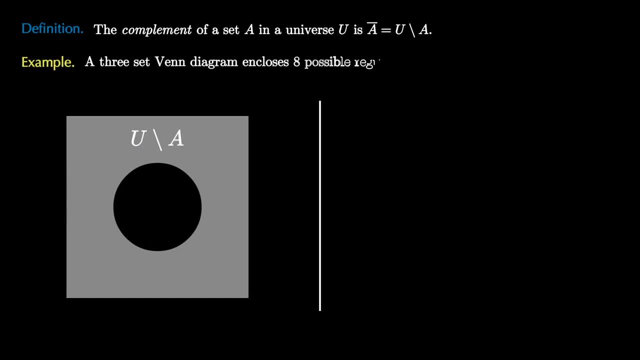 A. This is the set U set minus A. This is the set U set minus A. This is the set U set minus A. With this language we can draw a three-set Venn diagram and see that it encloses eight possible regions. So let's look at a universe U and inside let's have three sets: A, B and C. 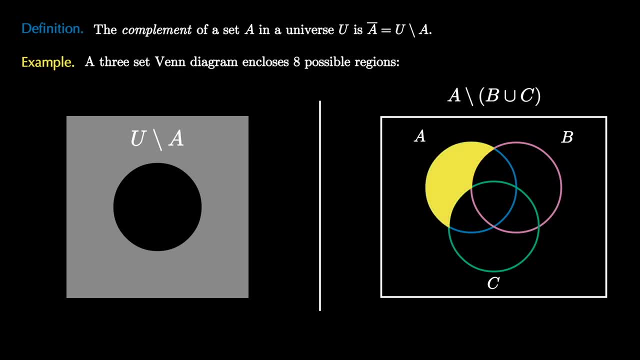 that possibly overlap. First we have the set of just the things in A and not in the union B. in C We also have the collection of things that are only in B and not in A union C. and we have the collection of things that are in the union B and not in A union C. 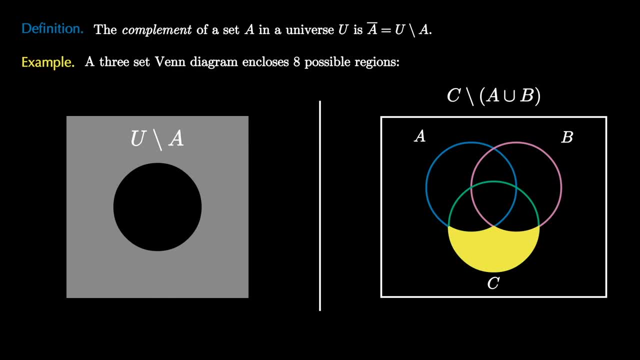 Two more areas. We have the set of things that are only in C but not in B and the addition of things that represent a mixture of elements is f in the rectangle. Or let's say that we have the set of things that represent a mixture of elements in C. 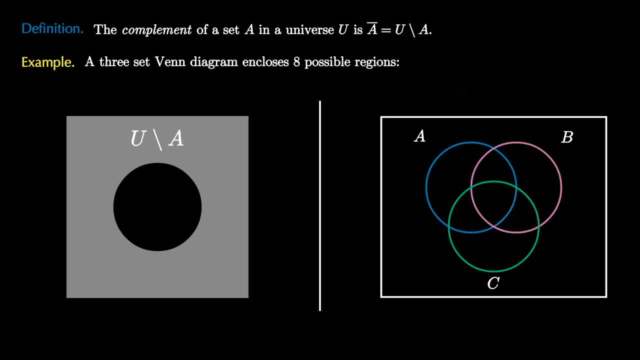 and not A union B. We can then look at the collection of objects in A and B, but not in C. This is a light rocket region at the top And we have three more similar regions. We have the things in A and C, but not in B. 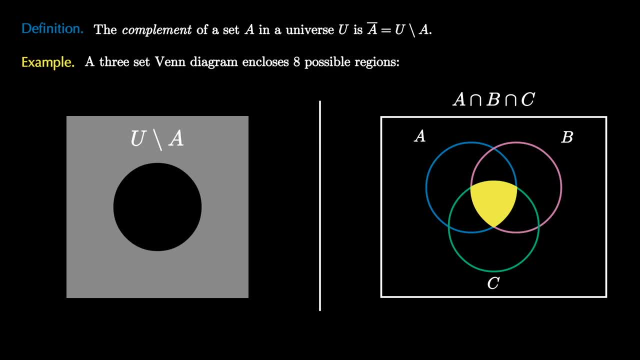 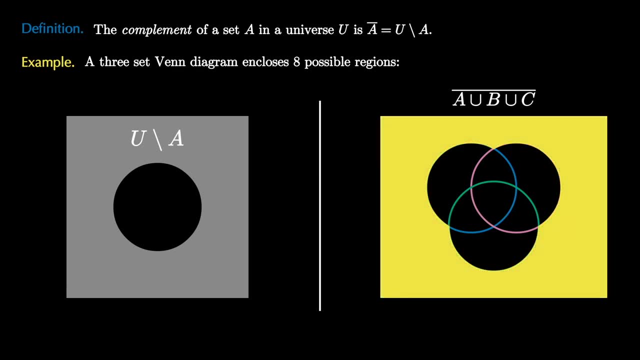 And then we also have the objects that are in B and C but not in A forms the rouleau triangle in the middle. That's seven regions, and so the eighth region, are the collection of things in the universe that are not in any of the sets or the complement of A union. 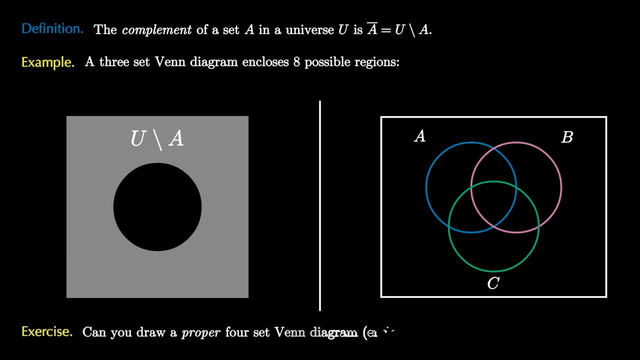 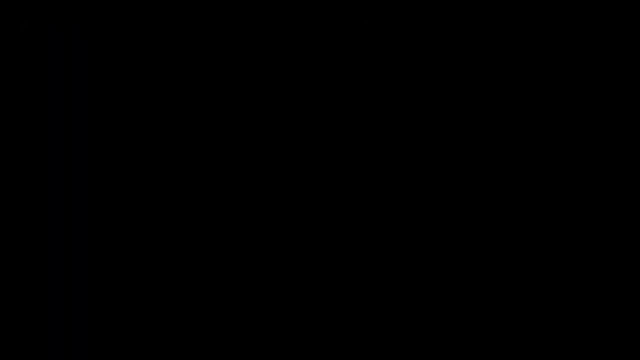 B, union C pictured here. Can you draw a proper four-set Venn diagram that will enclose 16 regions? To find a set-theoretic interpretation of the conditional connective, let's introduce the subset relation. We say that a set A is a subset of another set B if every element of A is also an element of B. 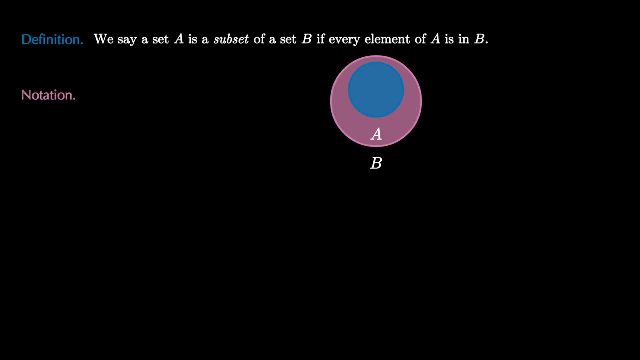 That means the Venn diagram looks like this, where A is completely contained in B. For notation we say A is a subset of B and we can interpret this logically. as for all x, if x is in A, then x is in B. so the subset relation is a direct translation of the conditional. 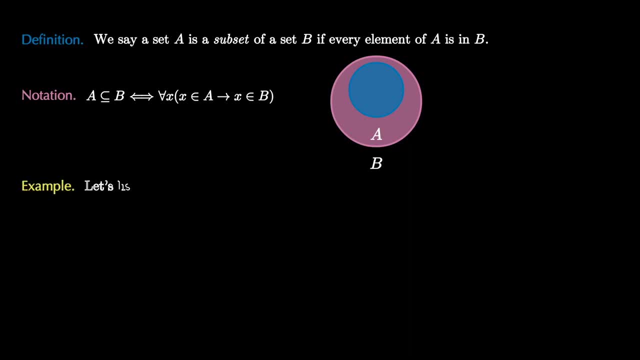 along with a universal statement. Let's see an example. Let's list all of the subsets of the finite set containing the numbers 1,, 2, and 3.. First we have the subsets with one element, like the one containing 1,. 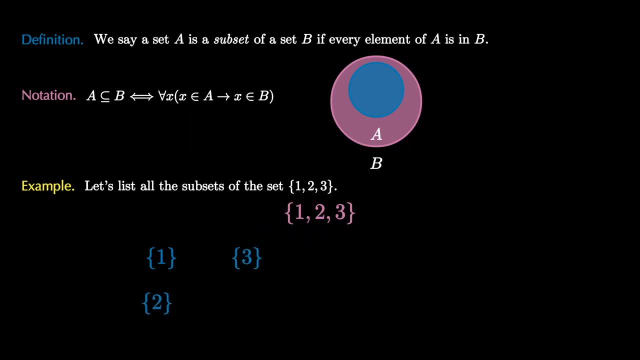 the one containing 2, and the one containing 3.. Then we have the subsets containing 1 and 2, the subset containing 1 and 3, and the subset containing 2 and 3.. And every set is a subset of itself by definition. so we have the subset 1,, 2,. 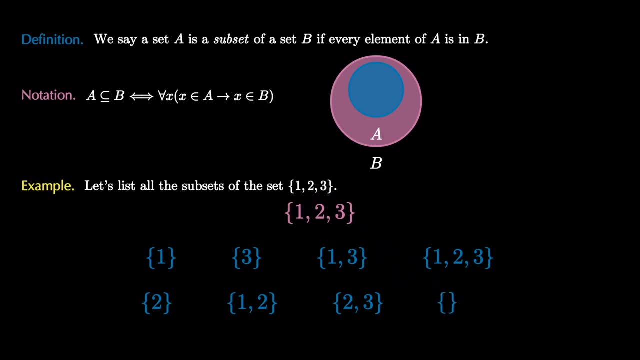 3.. It turns out there is one more interesting set, and that's the set with nothing in it, which we call the binary set and denote using this symbol here. So there are 8 subsets of the set: 1,, 2,, 3.. 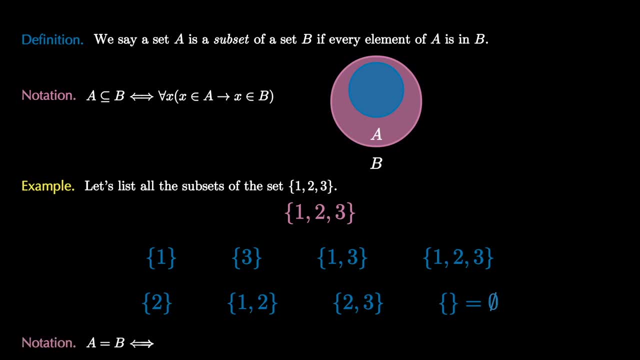 We can use the subset relation to define set equality. We say A equals B if, and only if, A is a subset of B and B is a subset of A. so the equality relation between sets is actually a direct translation of the biconditional connective. 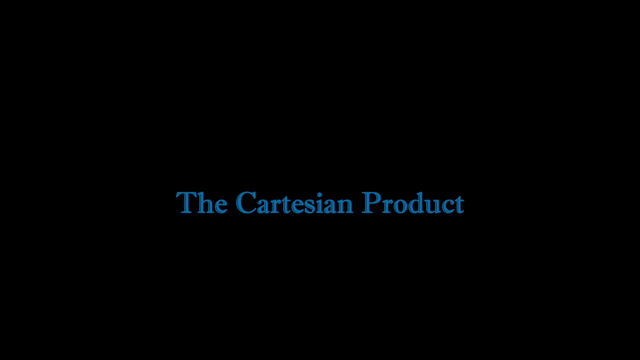 Let's finish this video with a final method of creating a new set from two sets known as the Cartesian product. Given two sets, A and B, which we'll show here as ellipses, we create the Cartesian product A times B as the collection of all ordered pairs of 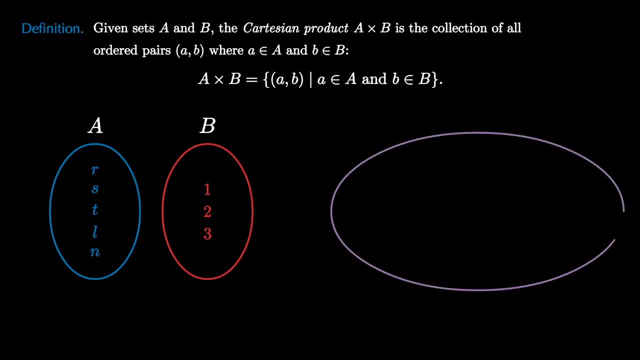 the form A, comma, B, where A is in A and B is in B. As an example, we've listed 5 elements in A and 3 elements in B. so to build the Cartesian product, we need to pair up every single element of A with every single element of B, And so we see. 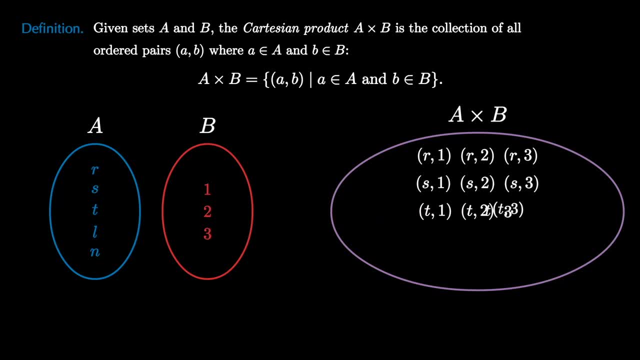 r pairs with 1,, 2, and 3, s pairs with 1,, 2, and 3,. t pairs with 1,, 2, and 3,. l pairs with 1,, 2, and 3,. 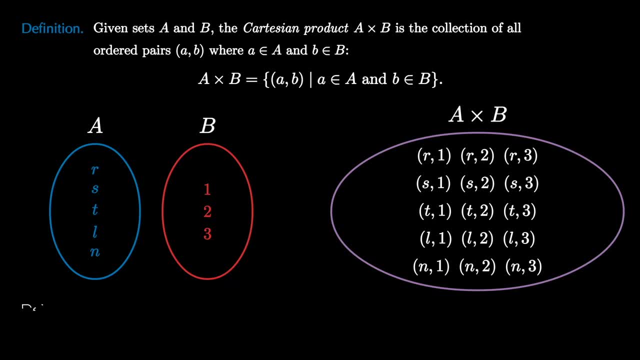 and n pairs with 1,, 2, and 3. This creates the entire Cartesian product. By the cardinality of a set A, we just mean the number of elements in the set A and we denote it by putting two bars on either side of the set A. I'll leave you with a final exercise. Can you find a formula for the?